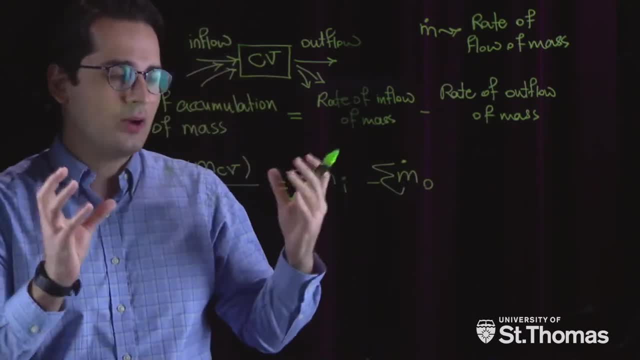 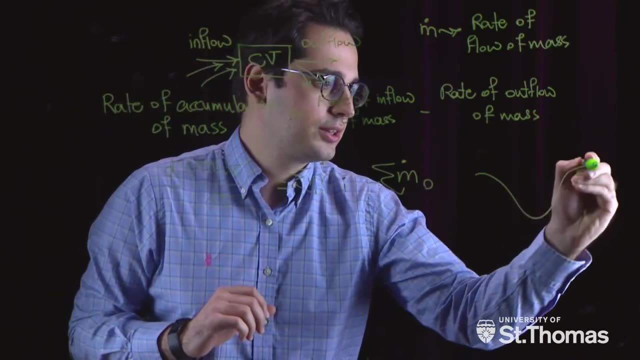 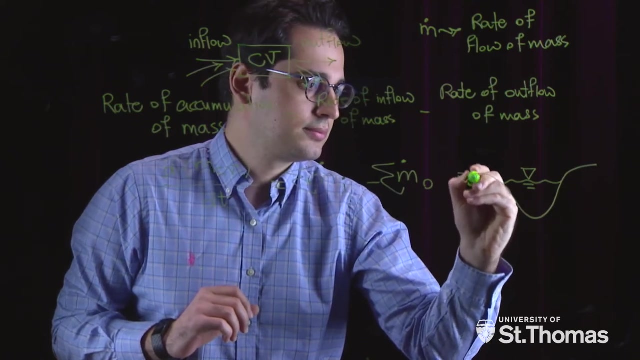 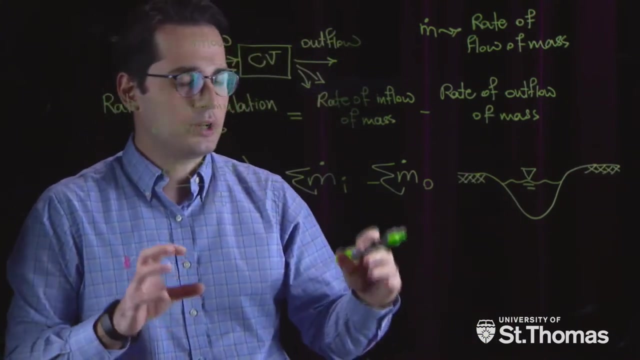 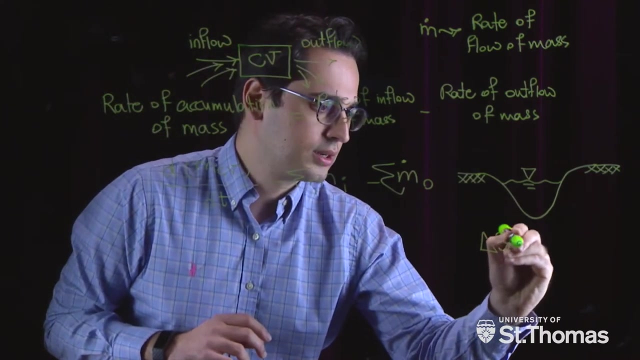 And c is the Sierra M d d, All right. So let's see, This is a um All right for this system. for this pond, if I want to apply the conservation of mass, the continuity equation it will be. changes in the storage of the pond is equal to inflow. 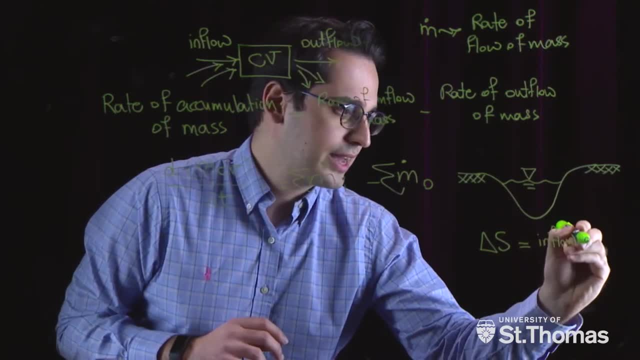 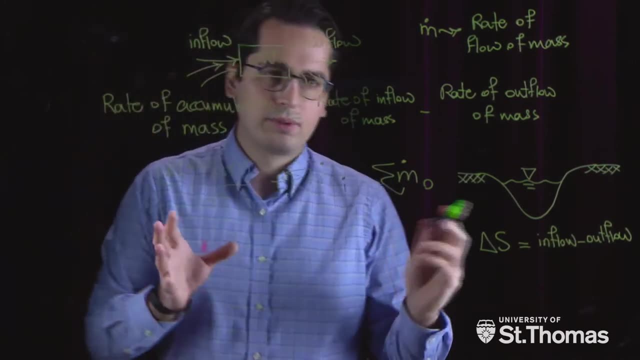 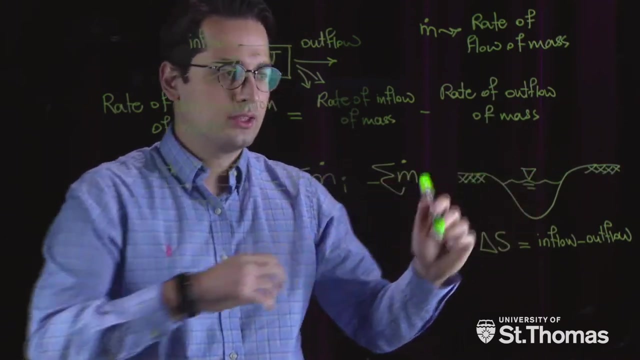 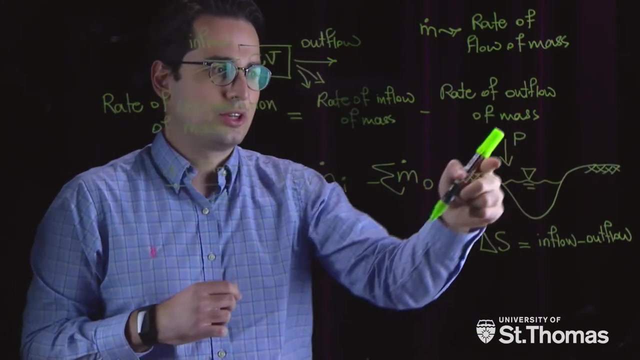 minus outflow- Perfect. Now, obviously, you're going to tell me that there are multiple inputs and multiple outputs for this system. Let's talk about those First of all. we know that there might be precipitation, And pay attention to the direction of the arrows that I'm having over here. 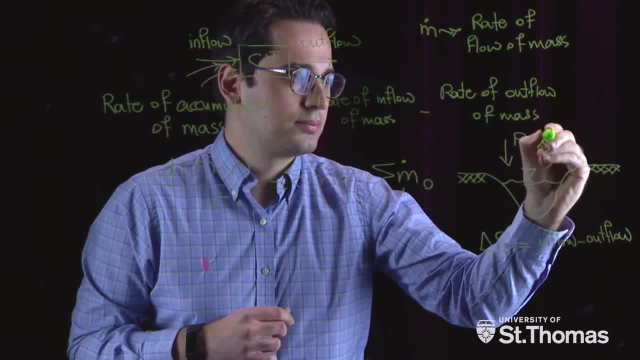 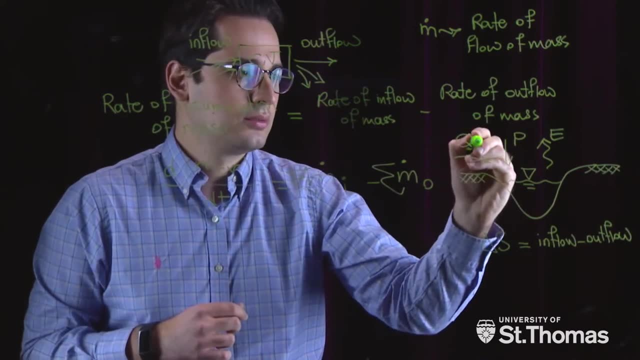 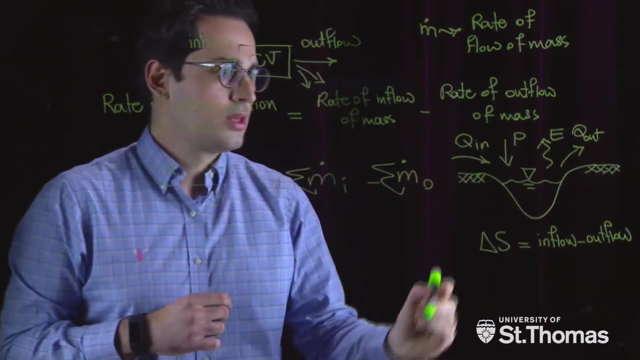 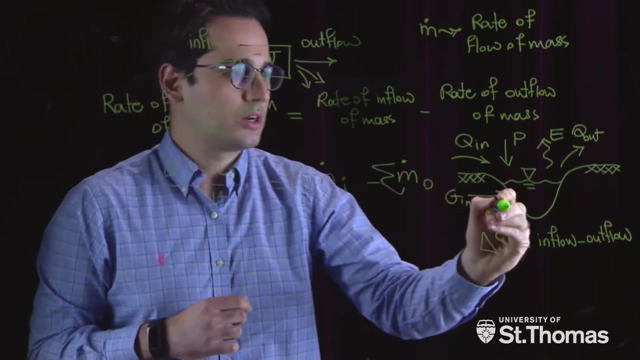 It might be evaporation out of this system. We might have surface runoff running off into the pond. We might have surface runoff out of the pond. We might have groundwater flow into the pond Or we might have groundwater flow out of the pond. 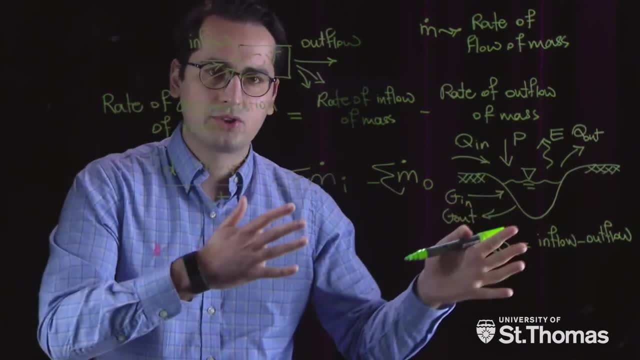 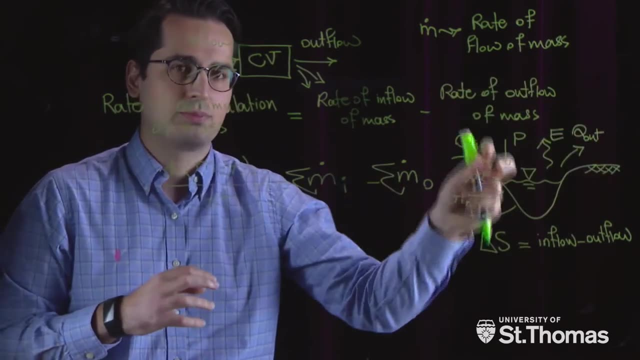 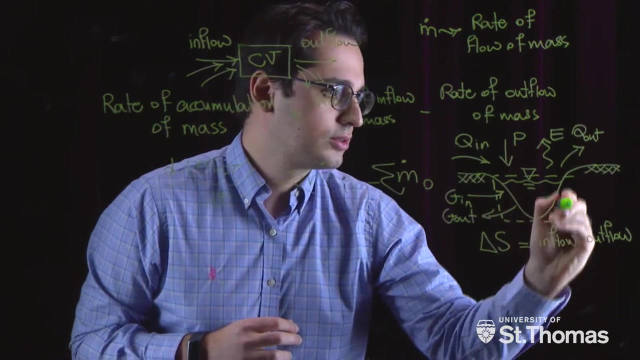 All right, so we have multiple inputs and also multiple outputs. If I want to write the continuity equation for this water resources system, this pond system that I have- and, by the way, the control volume in this system is over here- right? 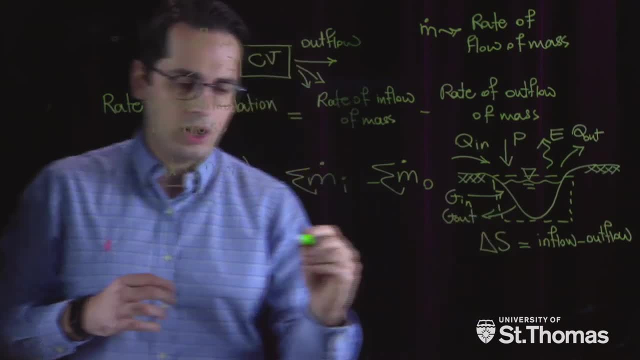 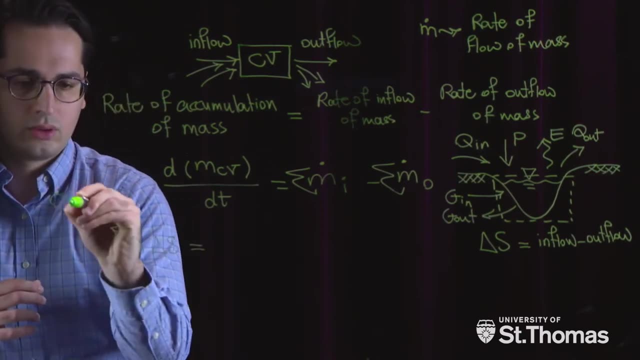 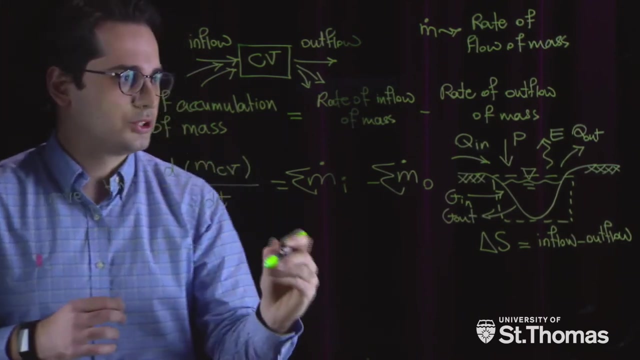 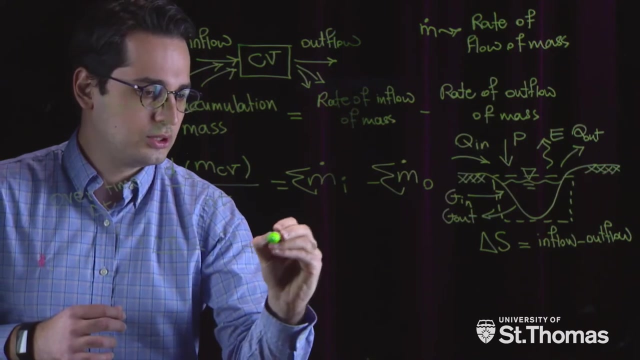 If I want to write the continuity equation for this, I'll be writing the changes in the system over time. delta T is going to be equal to. precipitation goes into the system. What else goes into the system? Q in surface runoff Plus groundwater in. 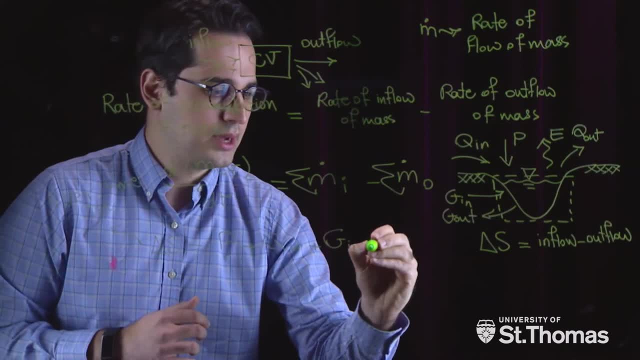 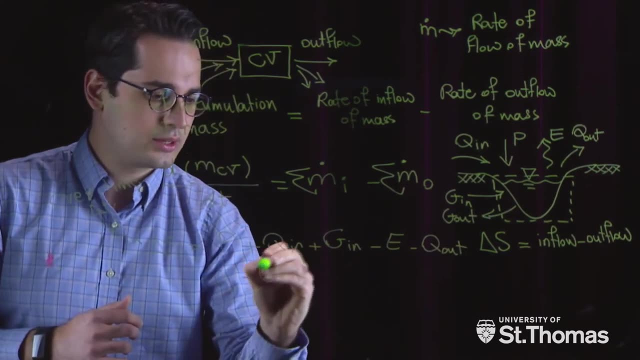 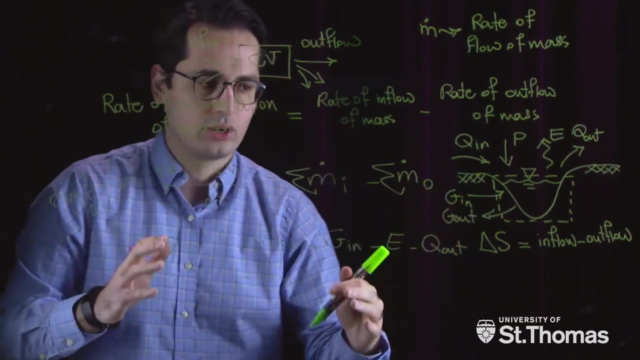 Minus all the terms that go out of the system. So it would be minus evaporation, minus surface runoff that goes out of the system, and then minus groundwater that goes out of the system. And this is your water budget or water balance equation for this system that you're talking about.